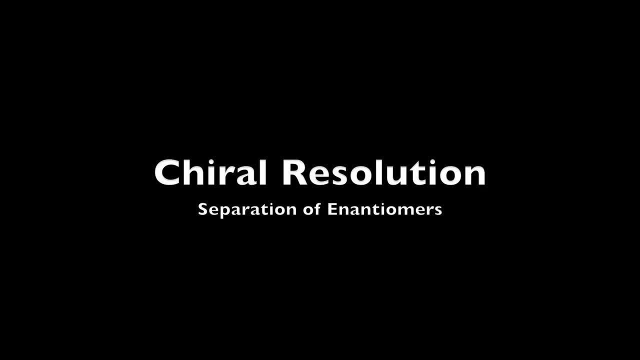 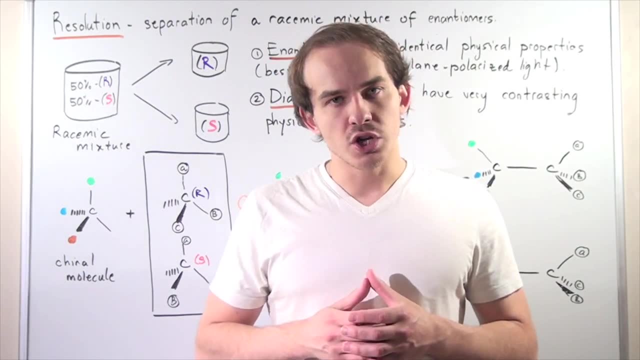 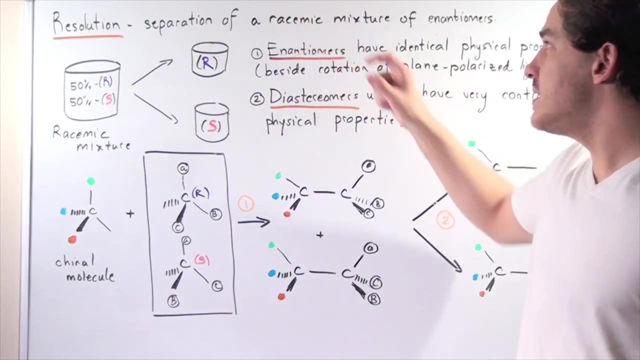 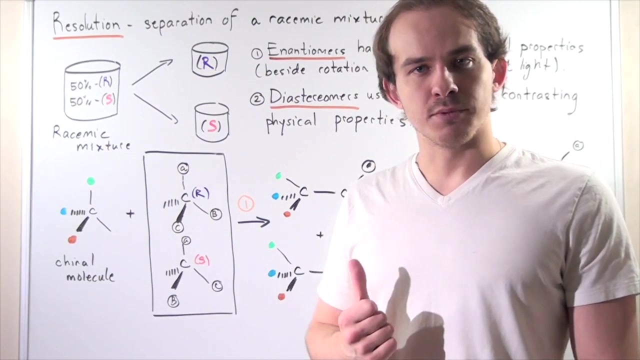 So in this lecture we're going to discuss a process in organic chemistry known as resolution. So resolution is the separation of a racemic mixture of enantiomers. A racemic mixture is simply a mixture composed of 50% of the R enantiomer and 50% of the S enantiomer. So let's 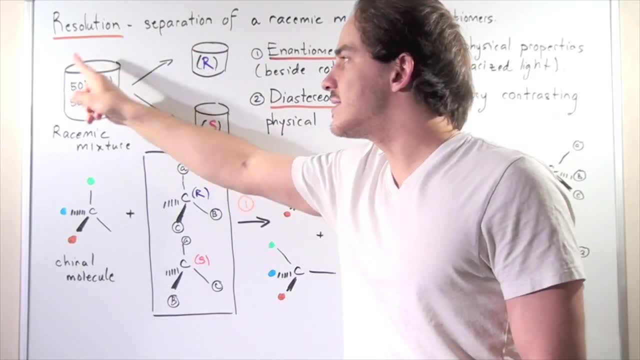 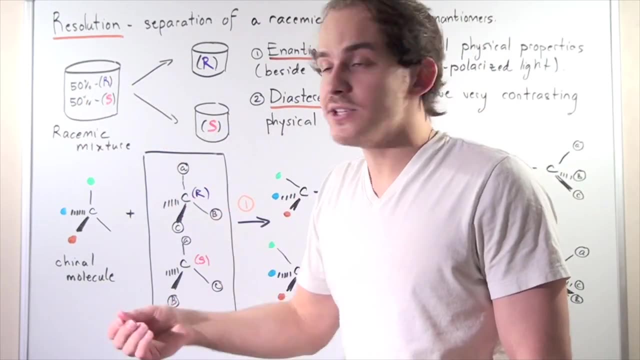 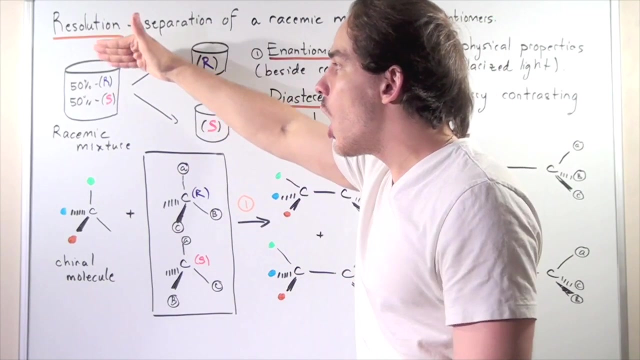 suppose I take my racemic mixture and place it inside a container. So this container contains 50% R enantiomer and 50% of its mirror image S enantiomer. So what resolution allows us to do is it allows us to separate the R from the S. So after resolution, we're going to have a container. 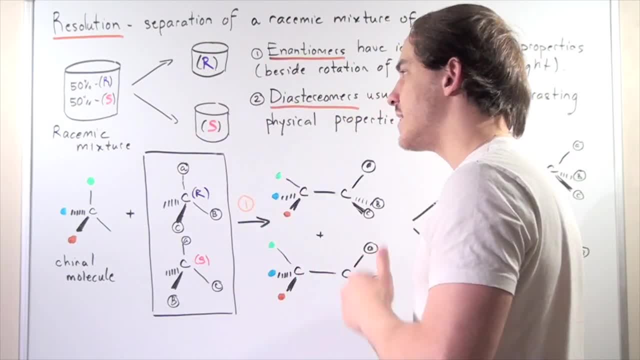 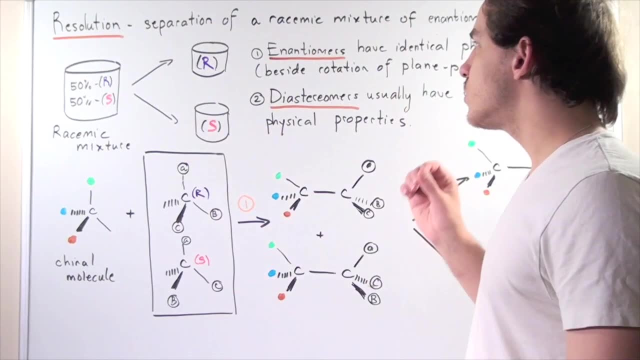 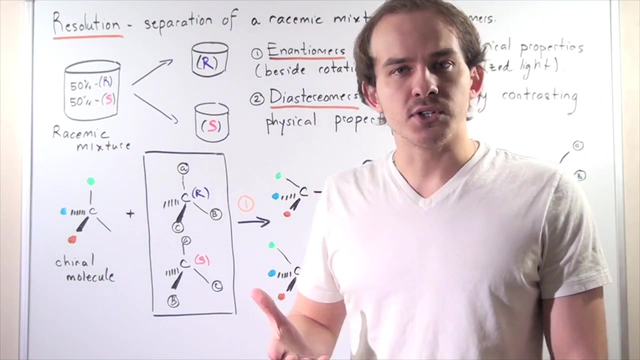 that strictly has R enantiomer and a second container that only has the S enantiomer. So before we discussed the steps of resolution, let's recall the distinction between anatomers and diastereomers. So anatomers are stereoisomers that are 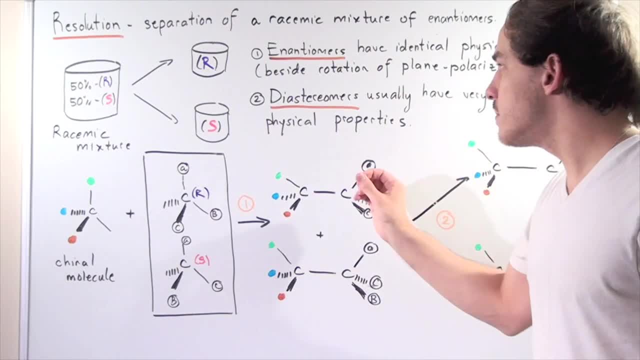 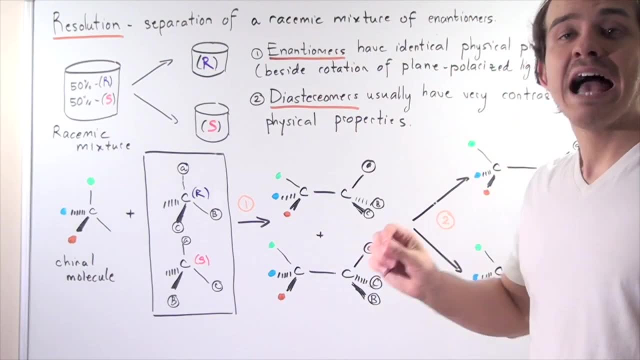 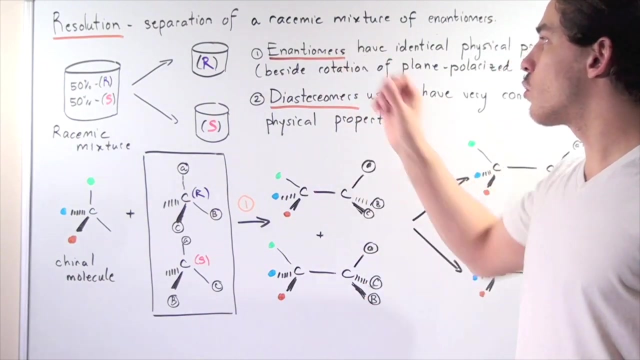 mirror images of one another, while diastereomers are stereoisomers that are not mirror images of one another. And anatomers have identical physical properties, So properties such as boiling point and melting point are exactly the same for anatomers. On the contrary, diastereomers usually have very 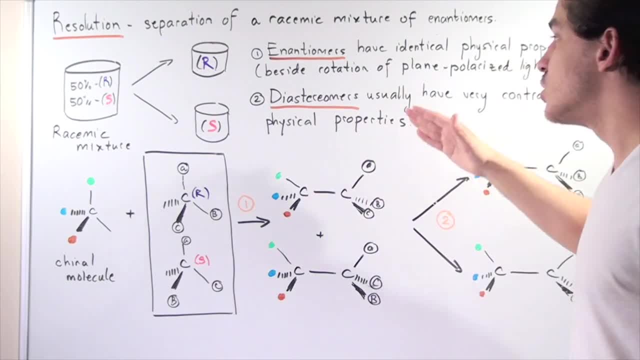 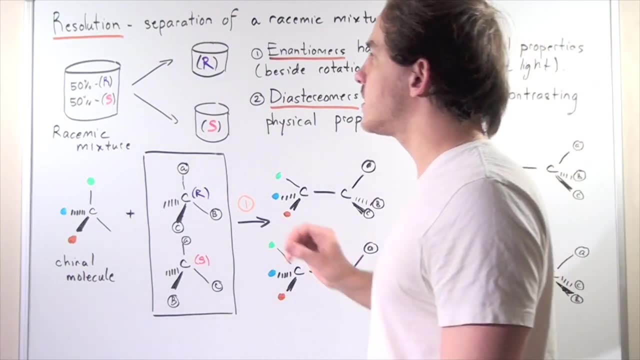 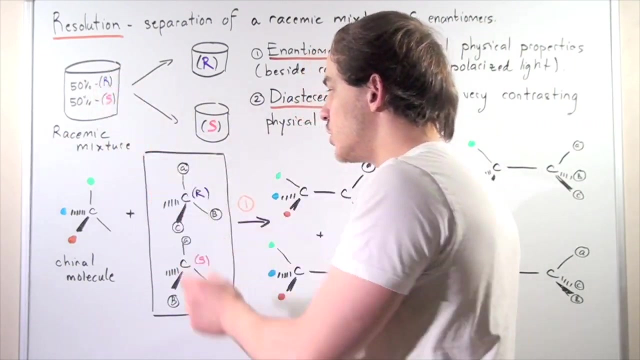 contrasting very different physical properties. So they differ in the boiling point or melting point of the compounds. So let's begin our discussion on the steps of resolution. So your first step is to take your racemic mixture. So here, 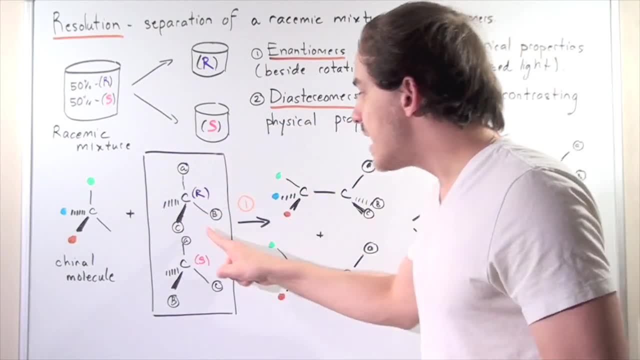 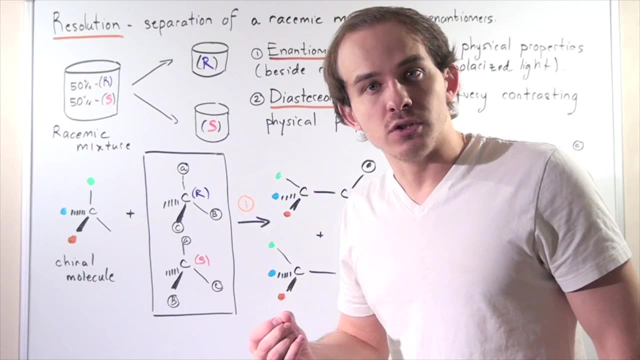 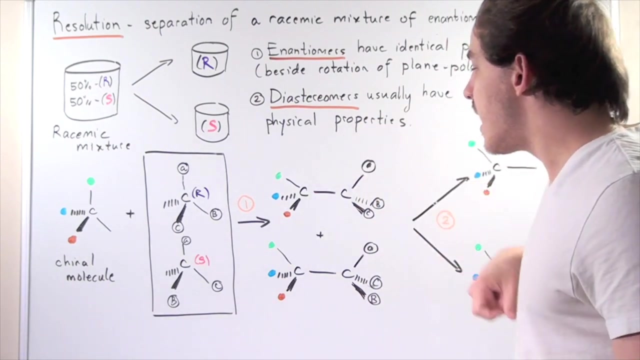 we have our racemic mixture. We have the R-anatomer and the S-anatomer And we mix that it or react it with some other chiral molecule. Now, when these react, they will form two different compounds. They're going to form this compound and the below compound. So when this chiral